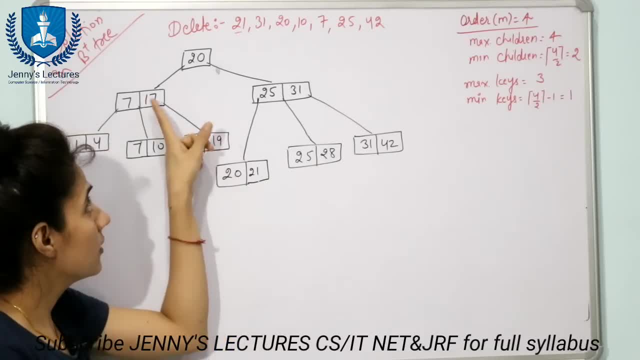 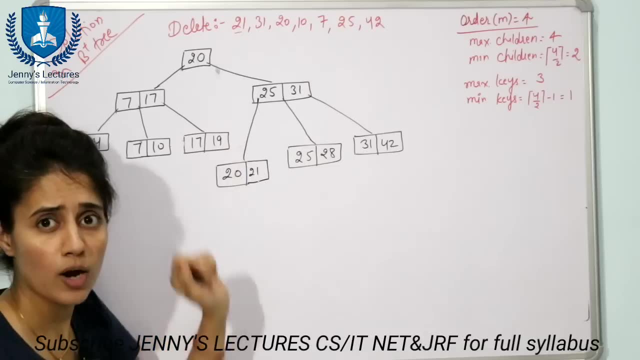 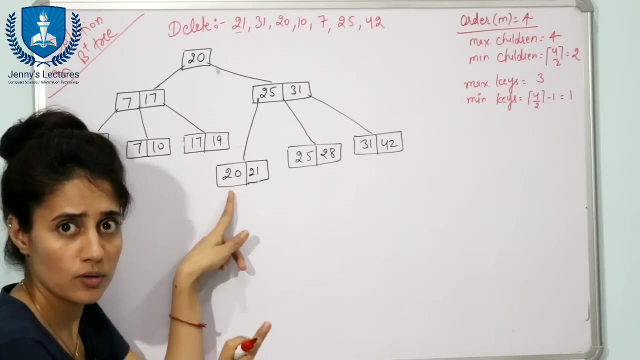 have to take care. one more thing also, because you have to check the indexes also. Maybe that data is present in leaf node also and that data is also in the index. So you have to delete the data from index also. Now, 21 is not present in the index, 21 is only present in the leaf node, fine, So 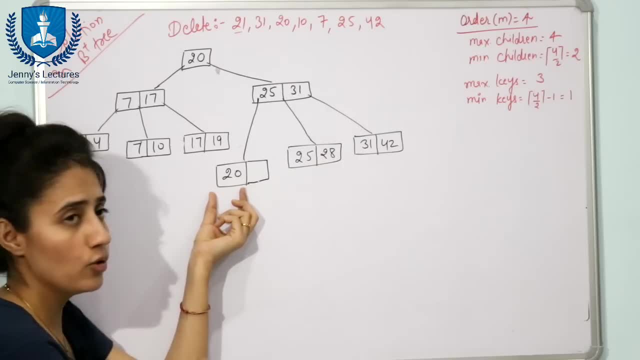 if you delete this 21,, you have to check the index also. So if you delete this 21,, you have to check the index also. So if you delete this 21,, then data is remaining, value is 1 and minimum key should be 1.. So this is still satisfying the property of B plus 3.. No need. 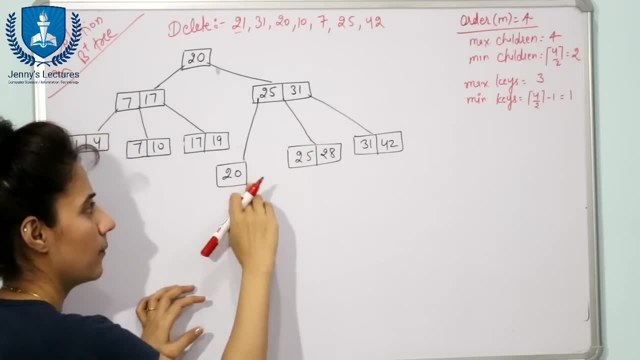 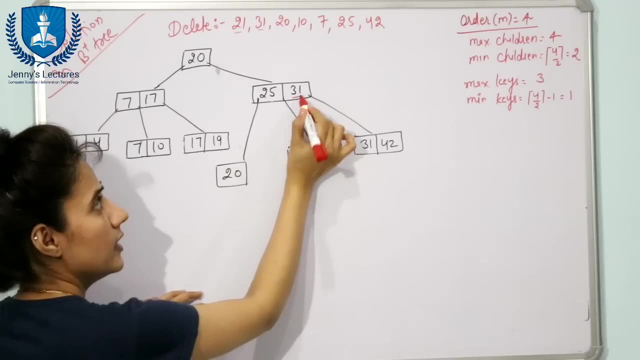 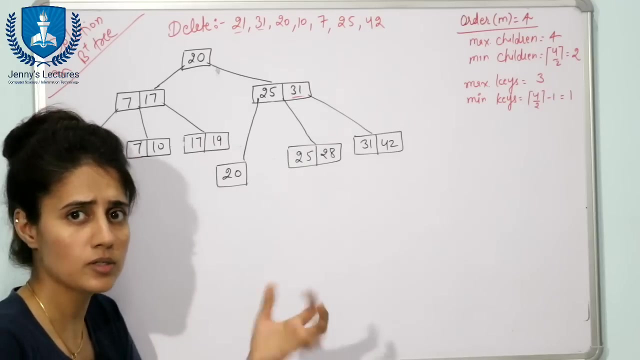 to do anything. This is the simplest case: Simply delete the data. Now next is 31. Search: where is 31? 31. See, here we got 31, but it is index. And now data is always present in leaf node. You are supposed to delete the data from the leaf node only because data 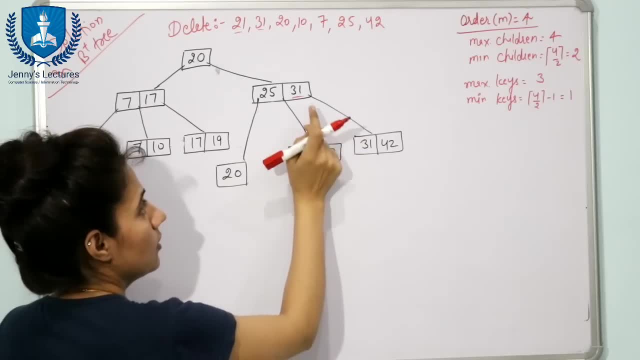 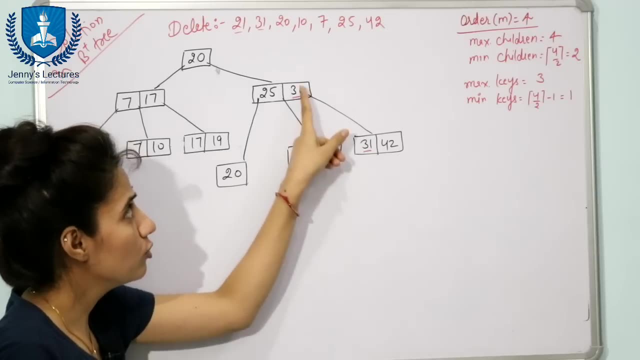 is only in leaf node. So now go to this side. Here you have to take care one more time. So on this right side here we got 31.. Fine, You have to delete this data from here also, and here also The index, associated index also. Now, if you delete this 31,, this 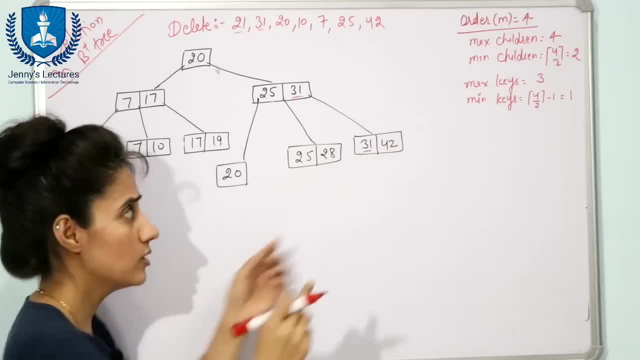 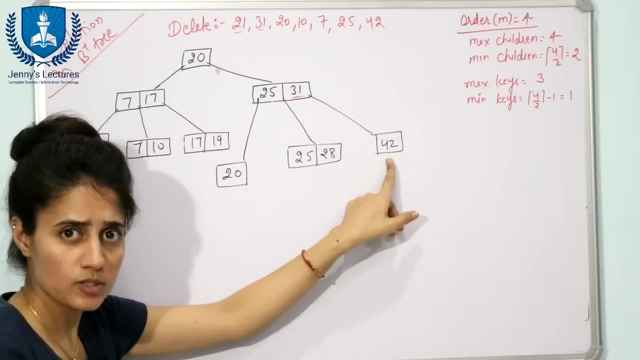 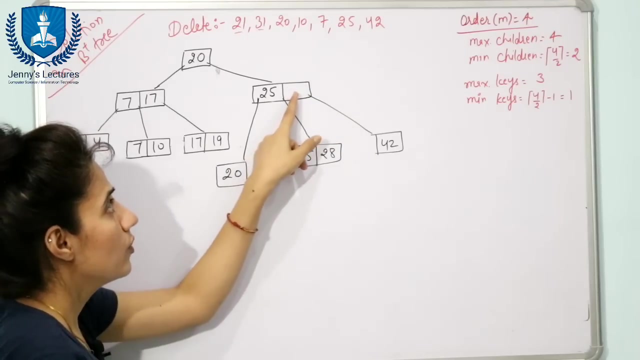 is the same case. This leaf node is having more than minimum number of keys, So simply delete this 31.. This is still satisfying the property of B plus 3.. Minimum tree is 1.. Now again, delete this 31 from here. Now what you will do. What index is this? What index? 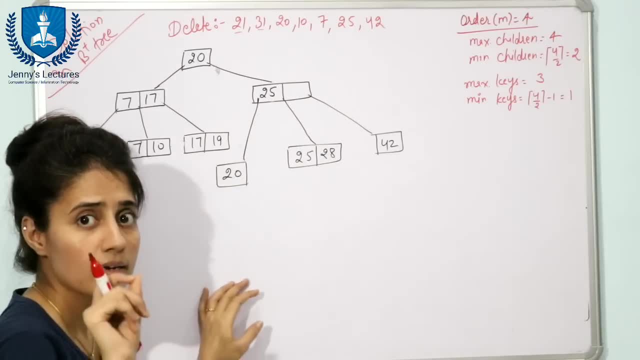 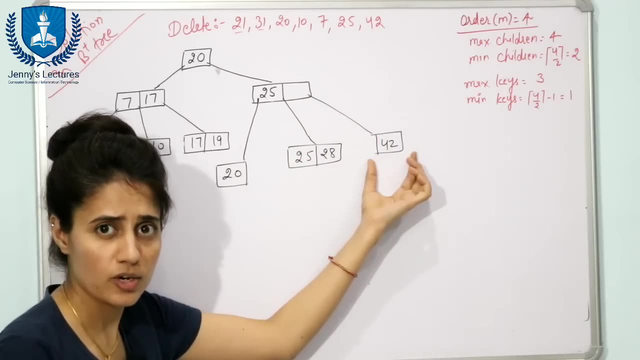 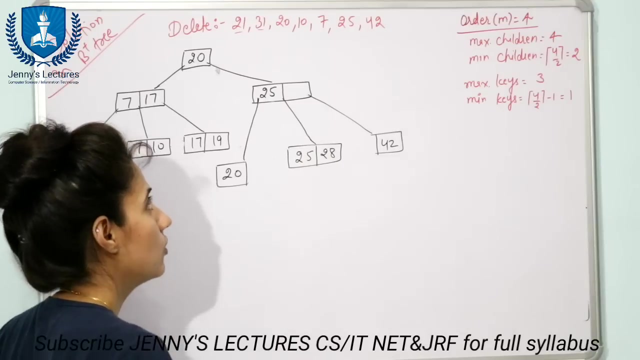 you will put here. fine, if this is the case, then then you will check out the right child- right child is this one- and you will take the minimum value from the right child, or you can say the first element of the right child. here we have only 42, so 42 would go here. so now, here you will write. 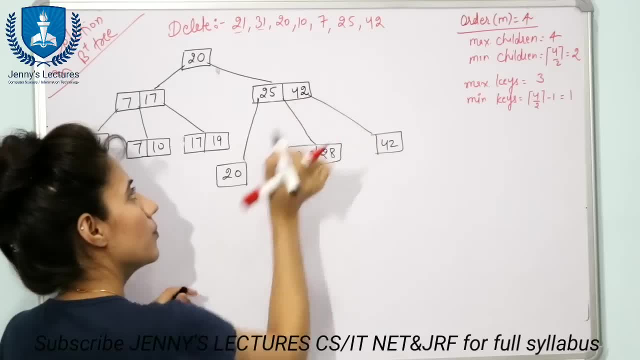 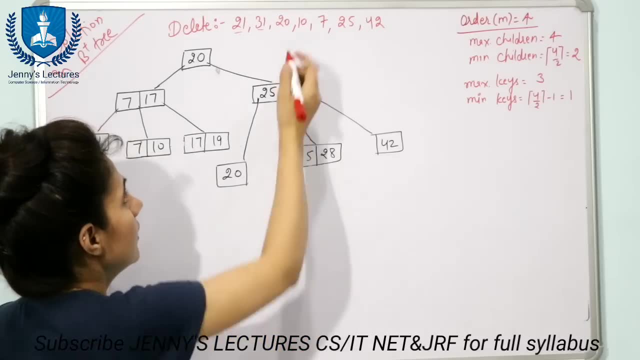 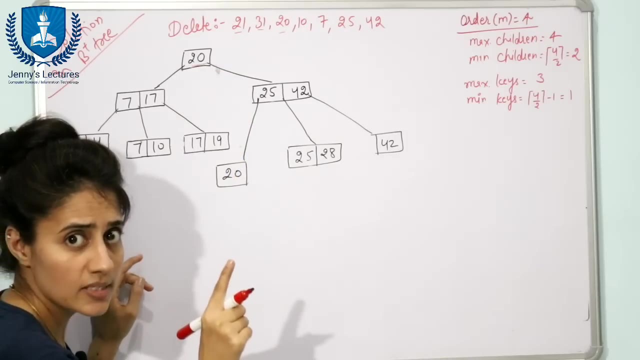 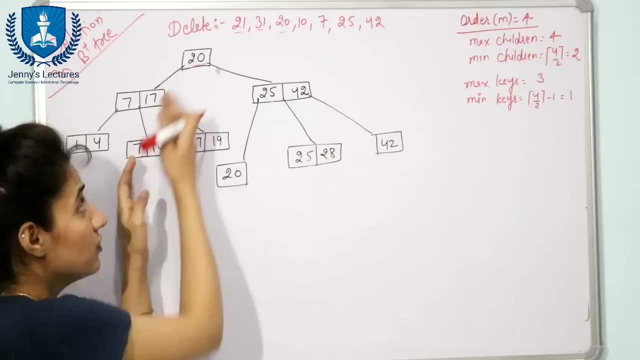 42.. so now this is the new index: 42. fine. next case: delete 20. now find where is 20. here we go 20, but this is the index. now see this: 20 is equal to this index and when we were creating the tree, we followed the rule that the left side value should be strictly less than this. 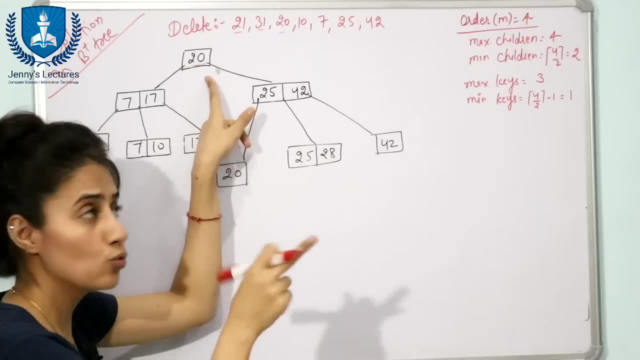 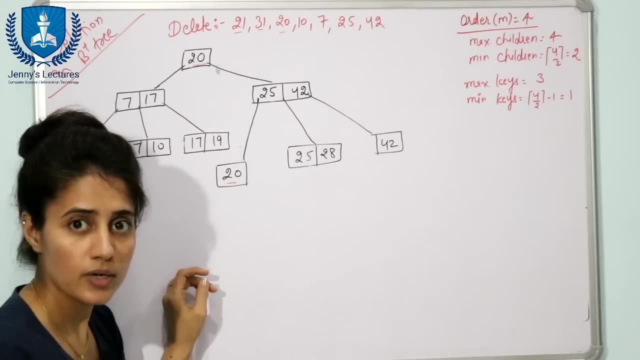 node and the right side should be either greater than or equal to this one. so 20 should be to the right side. so here 20 is less than 25. so here we go, 20. fine, see, in some videos you will find out that they follow the rule that to the left side you can have the values. 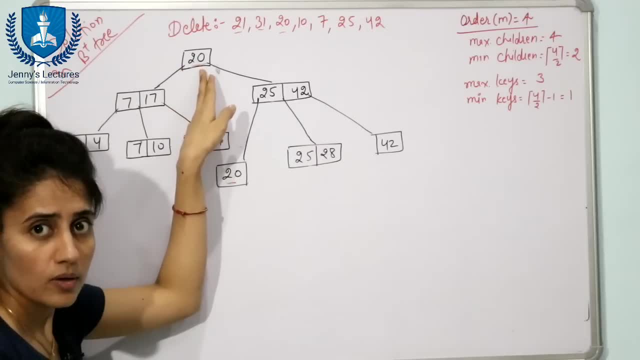 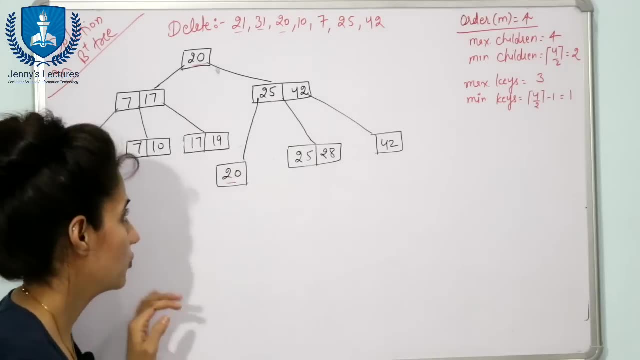 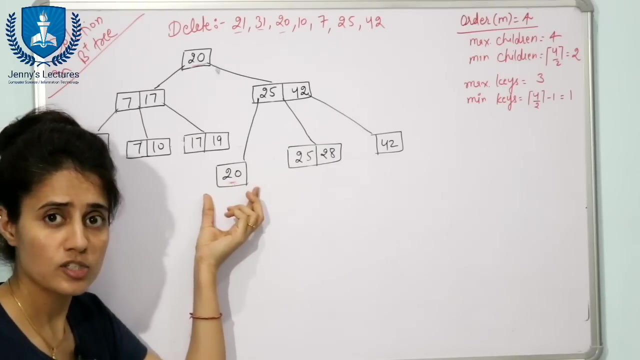 either left, either less than or equal to this node, and to the right side, value should be strictly greater than this node. fine, so you can follow either approach to create a b plus tree. now you have to delete data from a leaf node now. now the second condition: this leaf node is having only minimum number of keys, and if you delete this, 20. 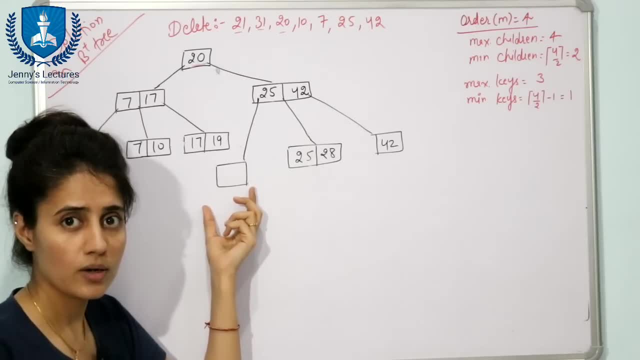 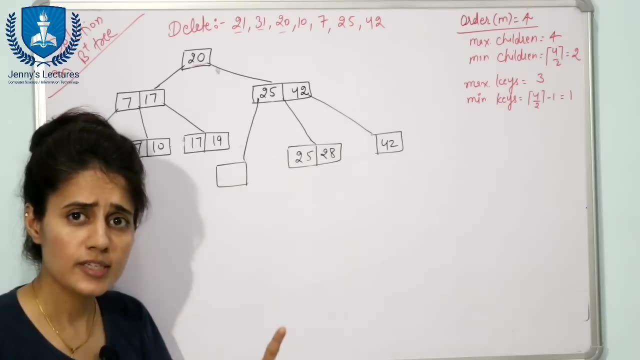 then this node is having zero key and that is not possible. this is violating the b plus tree property. now, what you will do now, first case is either it can borrow from its left sibling, or second case is it can borrow from its right sibling, or you can say from immediate left node or immediate right. 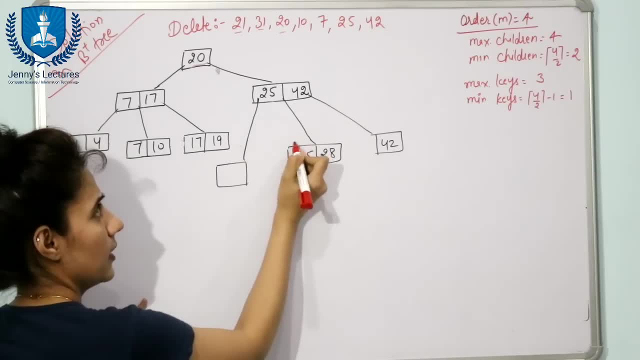 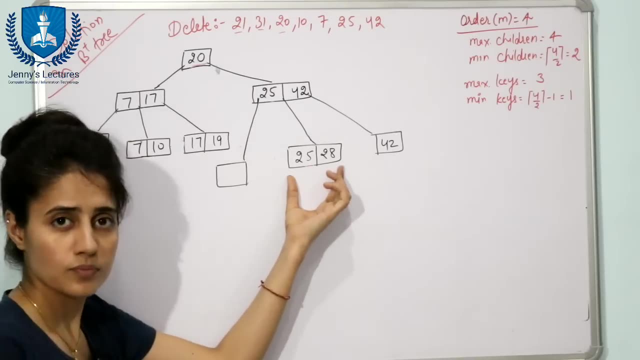 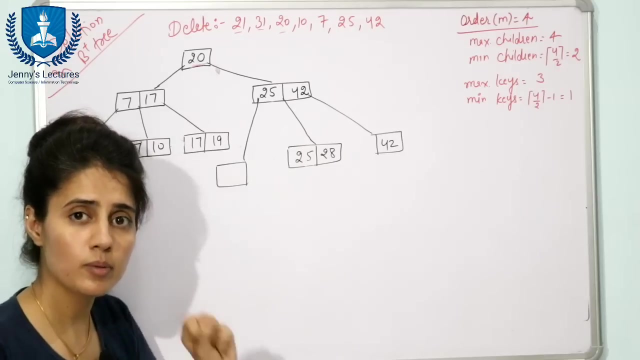 node. fine, now here we have right sibling. fine, now check. the right sibling is having 25 and 28 2 values. see, this node can borrow key from its siblings if that sibling is having keys more than minimum number of keys. so it will ask to its sibling: can you give me one key? 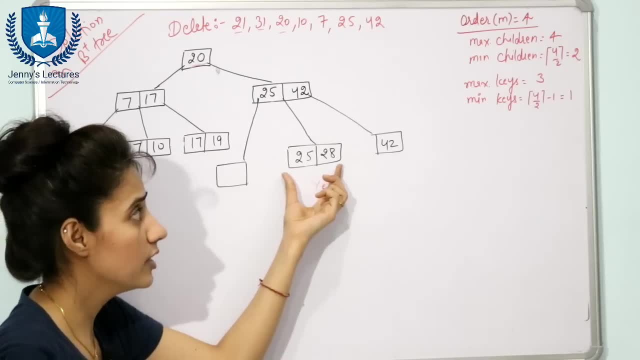 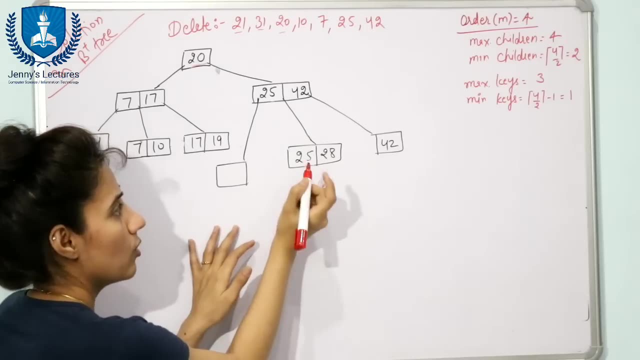 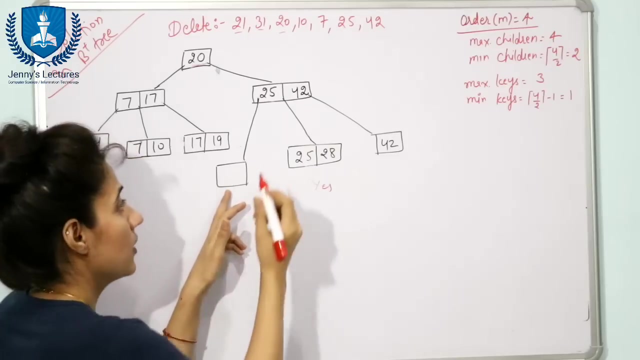 this will say yes. i can give you why it is saying yes: because it is having keys more than minimum number of keys, so it can give one key. still, it will have one key left. so now this: borrow this key from right, sibling through the root node, as you have discussed in b tree. 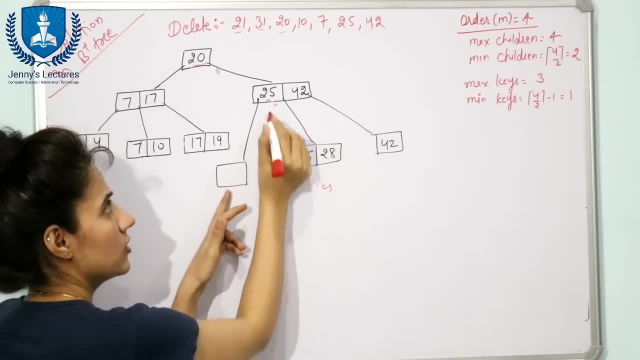 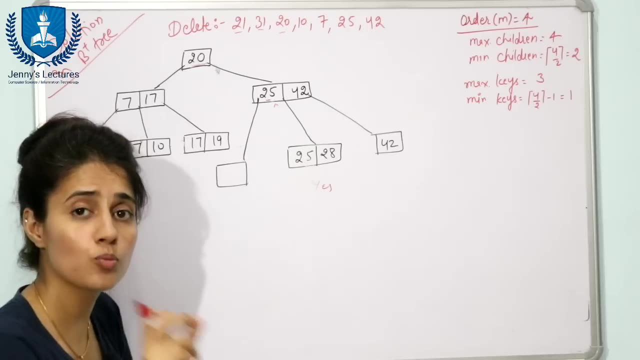 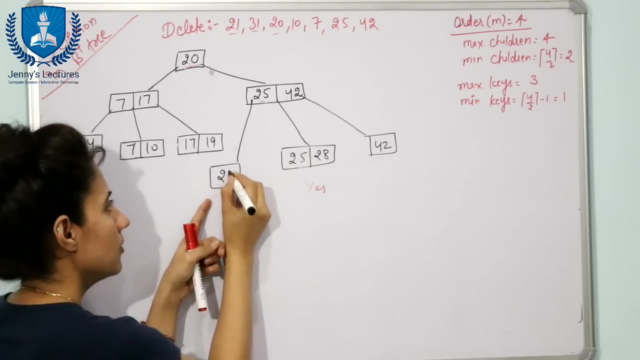 so now through the root node, here we have only the index, so it will borrow from here the minimum. from its right sibling it will borrow the minimum key, the smallest key. you can say smallest is 25, right, so here you will write 25 because we have borrowed 25 from here. fine, so now we cannot write 25. 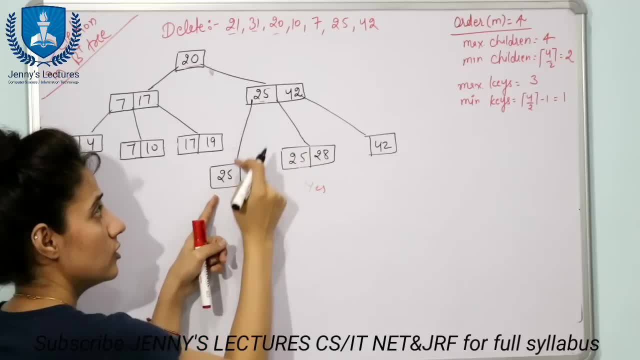 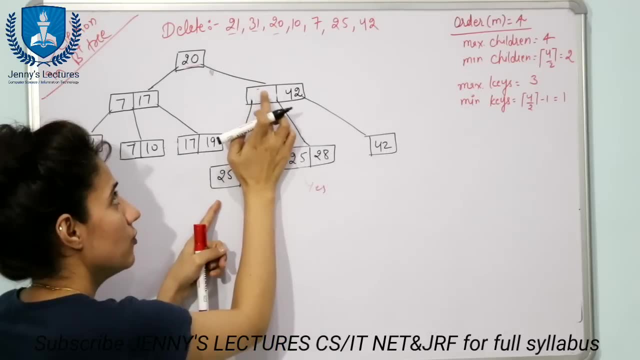 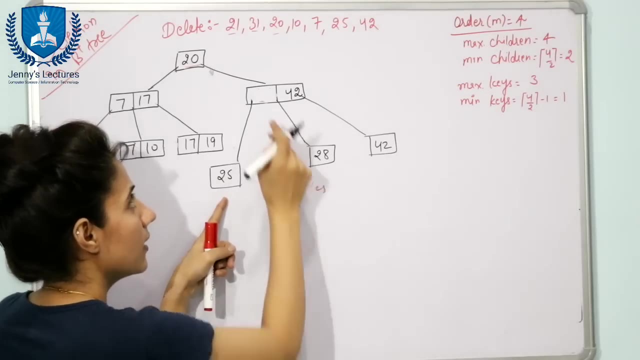 here we can see, the value to the left of this should be strictly less than the value present here. only so here you will not write 25 we have borrowed because 25 here only so we will delete 25 from this node. and what should be the value here? the value, the minimum value from here should be: 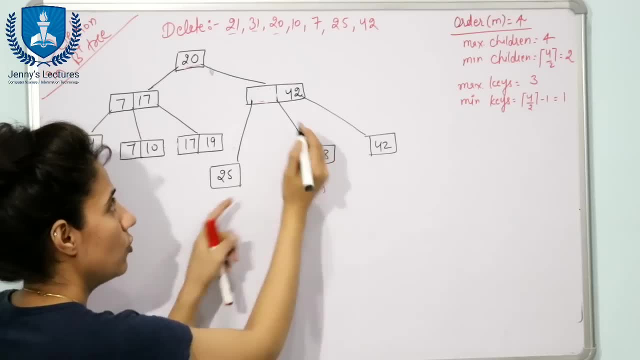 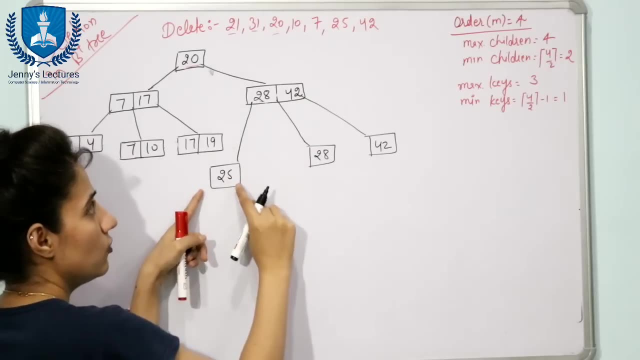 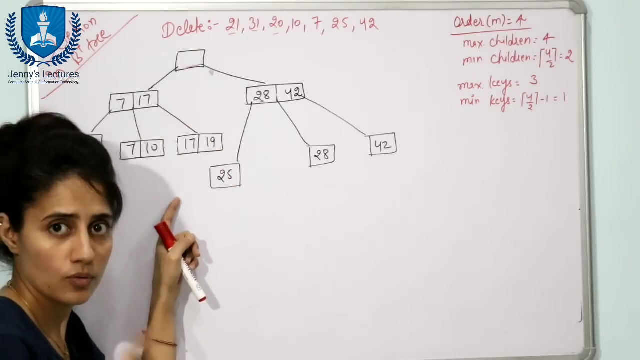 from its right child. right child is having 28, one value only, so we will write 28. now index become here 28. so now next is we deleted this 20 from here. we are also having the index also, so you have to delete 20 from here also. fine, now next thing, what you will do is see, you will put here. 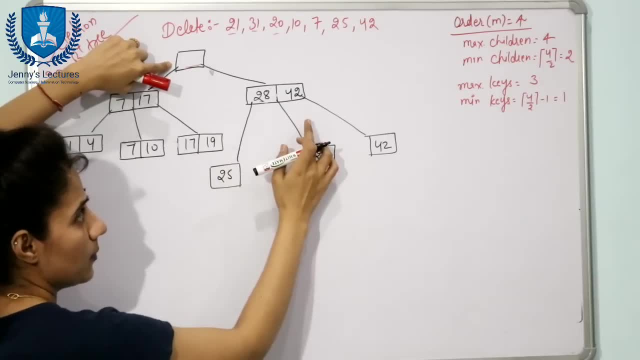 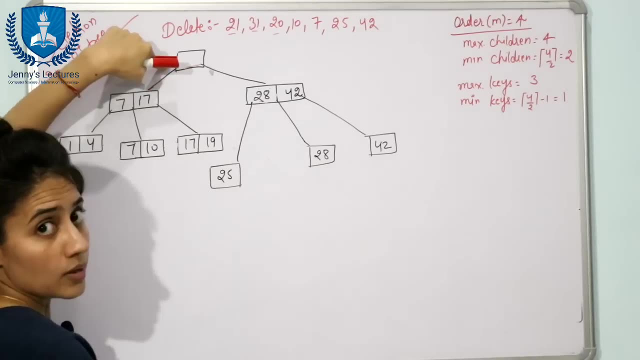 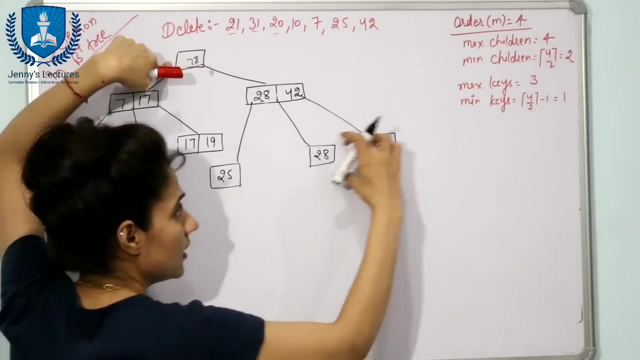 what the minimum value from its right, right sub tree. so here are the leaf. so minimum value should be 20, so minimum value out of these is 25. say, please do not check from here- that minimum value is 28, so write 28 here. no, because the data is always present in the leaf node. these are just 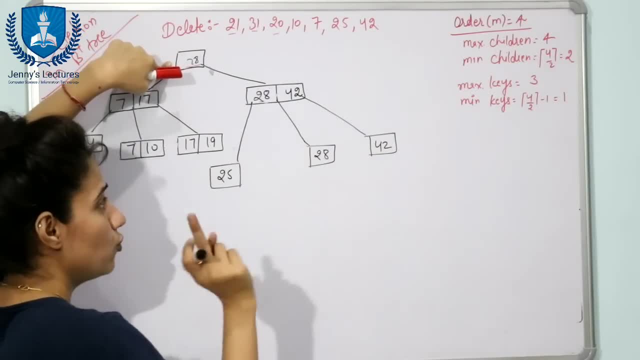 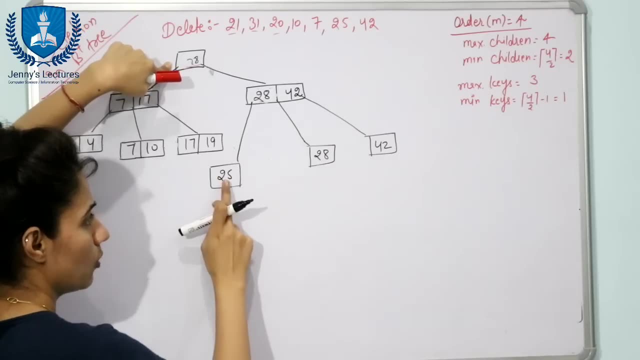 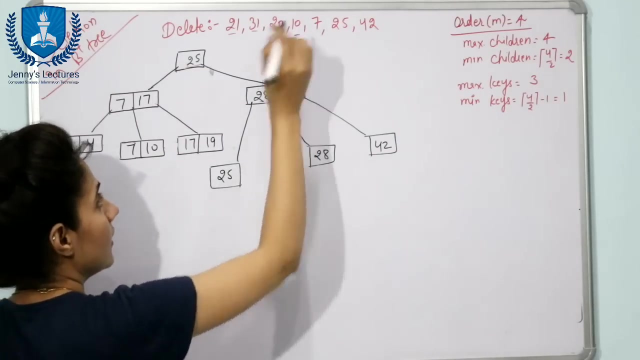 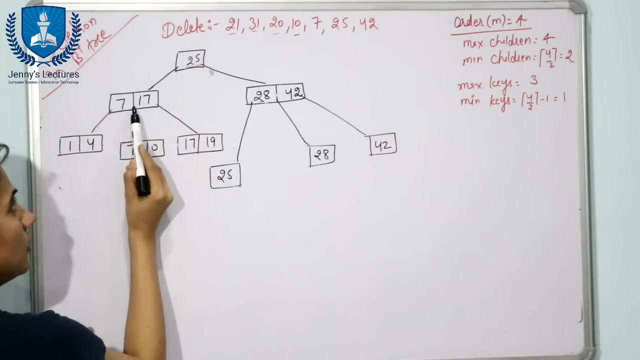 the indexes. so we are going to place, we are going to find the minimum value, the smallest, from the data only. so data is in the leaf nodes. out of these three, smallest is 25, so we will write 25 at here, only fine now. next is 10. now find where is 10. 10 is less than 25. go to the size. 10 is greater than 7, less than 17, so go. 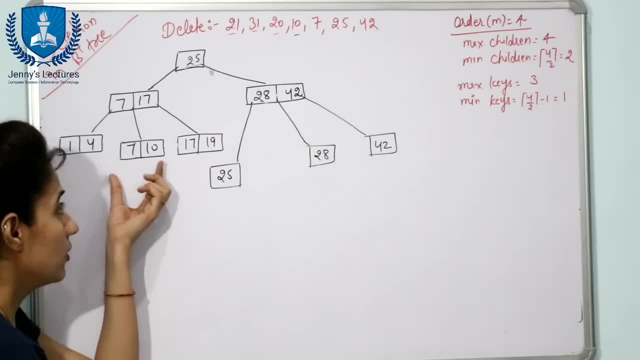 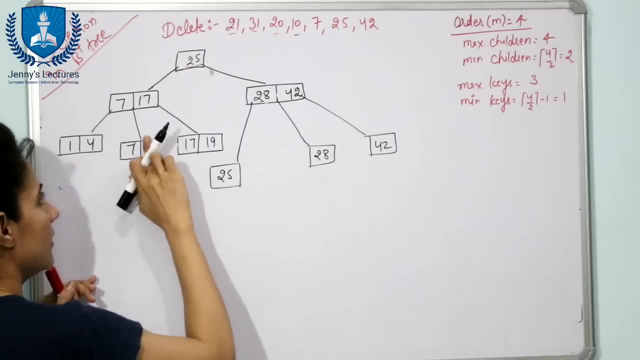 to this side. now, here we got 10. the same thing, the same case. we have this. this leaf node is having more than minimum number of keys, so simply delete this. 10 and indexes are not having any value. 10, so fine. so here we have only 7. now to the right of the 7. fine, next, delete 7. now find. 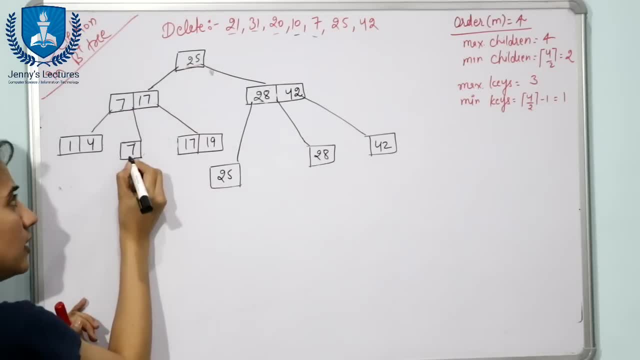 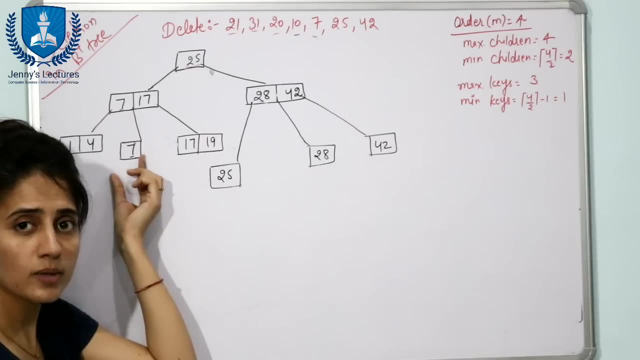 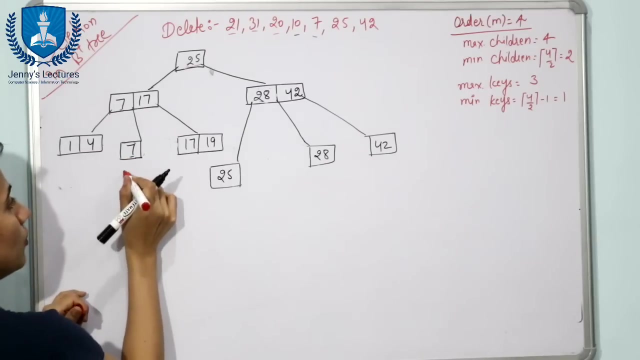 where is 7 less than this? here we got 7 and here the data is here and this is the index. okay, now, if you delete this 7, then this is violating the B plus 3 condition, because this leaf node is having only minimum number of keys and if you delete this one, here we go here, the node would be null, and that is. 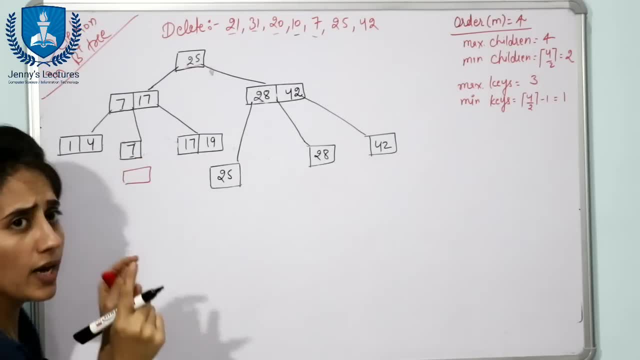 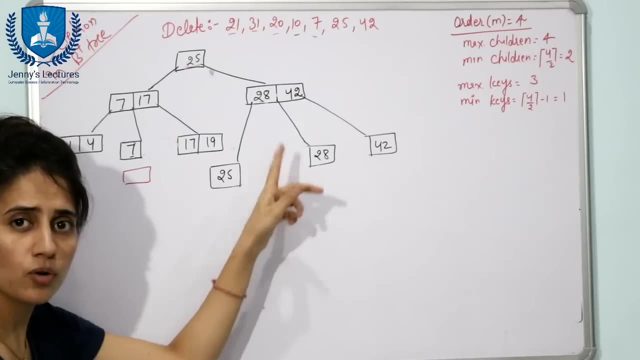 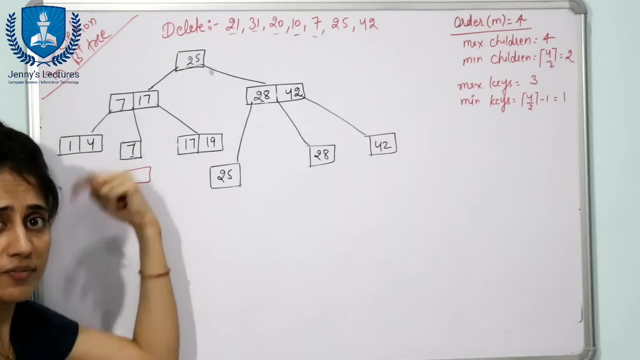 not possible in B plus 3, so now it will ask it will borrow data from its left sibling or its right sibling. so now, here I am going to discuss the case where this, this node, is borrowing data from its left sibling. see, it can borrow either from its left or from right, because both are having both. 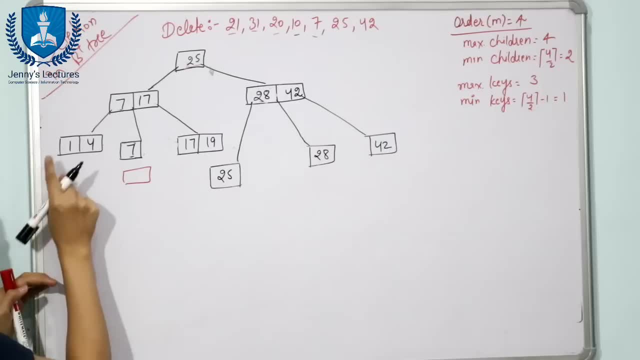 siblings are having more than minimum number of keys. so here I am going to discuss from the left first of all. it will check to the left and it will ask: can you borrow me one uh key? and it will say yes, why so? because it is having more than minimum number of keys and it will borrow through the 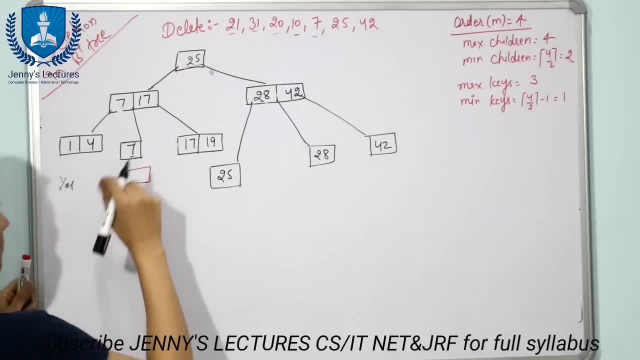 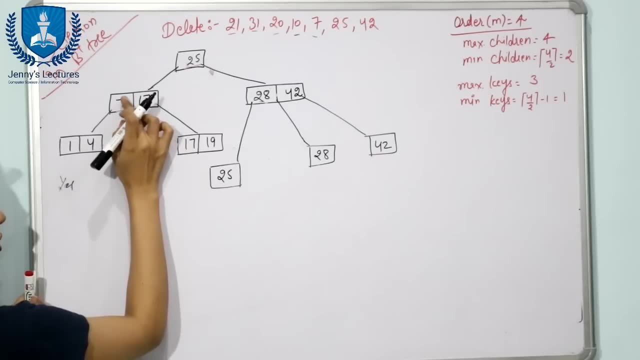 root node only. fine. so now here we have deleted the seven and from here also you, you have to delete the seven. fine, so this: if you are borrowing from the left sibling, then the, then the maximum value would be borrowed. here we have four, then four would be borrowed through the root node here. 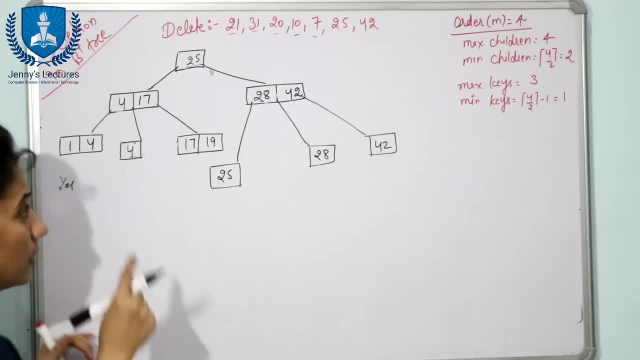 we will write four and here also you will write four. fine, and from here you will delete this four. so this side you will have only key one. fine, see why we have written this four. this value is always the minimum value from its right child, and right child is having only four. so here you. 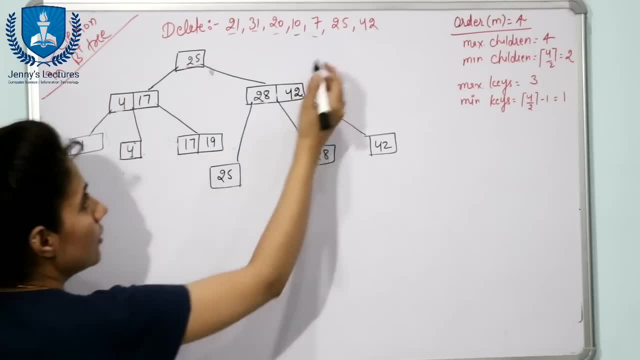 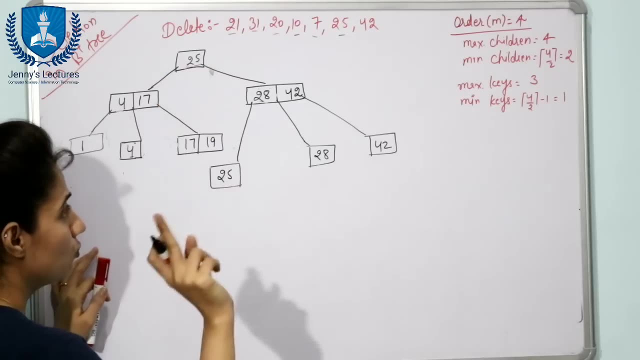 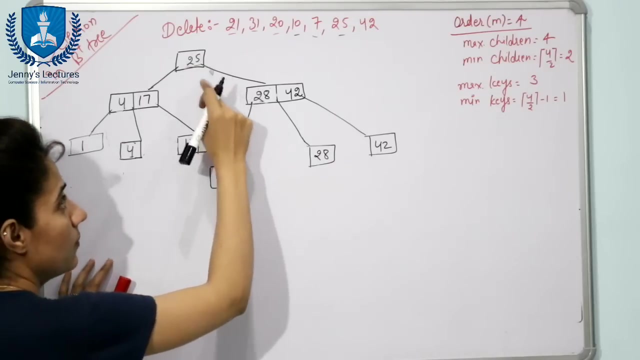 will write index should be four only. so now. next you will delete what 25 now find. where is 25? here we have 25, but this is the index. go to. we have to check for the data also. now 25. the data should be to the right side of this one. fine, so now 25 is less than 28. so here we. 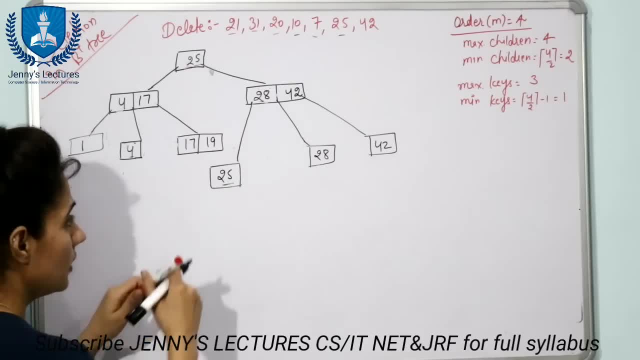 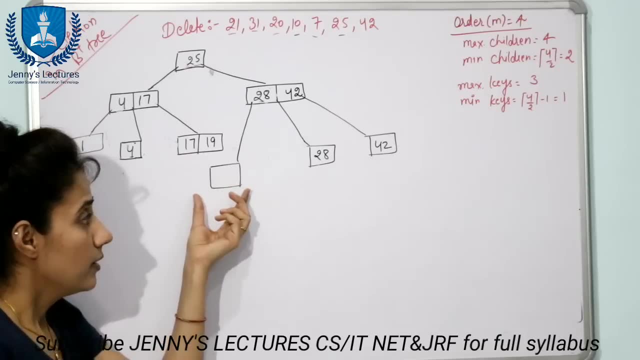 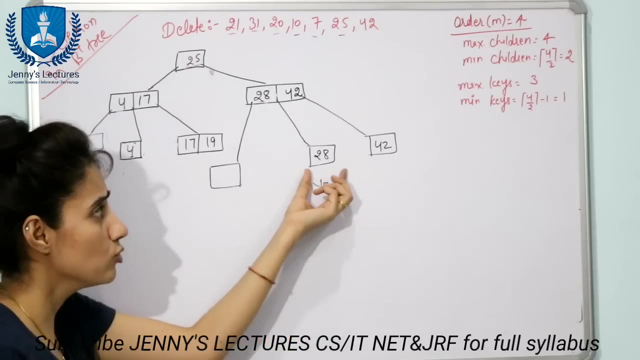 got 25.. now see, if you delete this 25 from here, fine, now it is having zero key only. so it will ask to a sibling, can you give me one key? and it will say no. why so? because it is also having minimum number of keys. so now we cannot borrow. 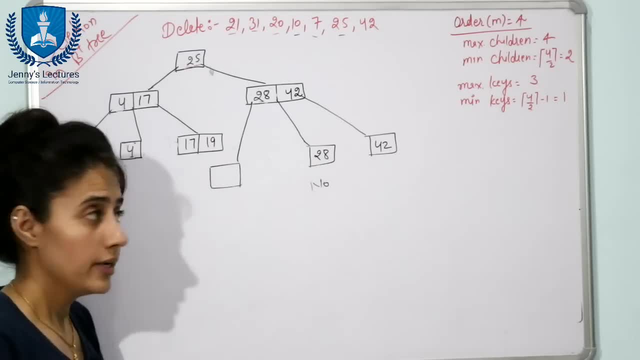 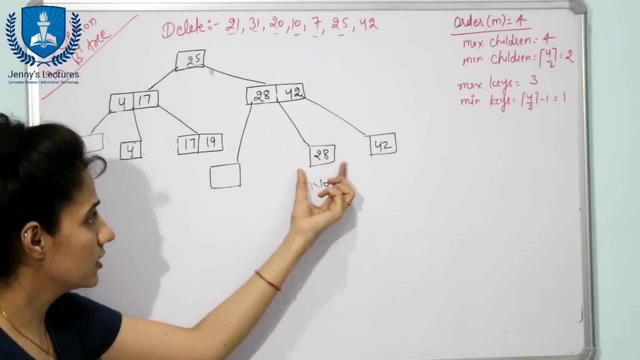 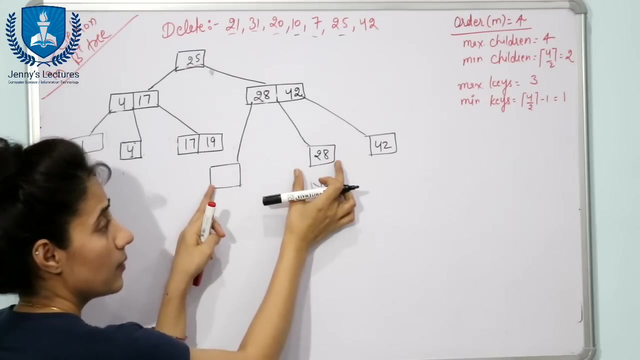 so next case is merging of the node. now this node would be merged either with its left sibling or right sibling. now in this case we have its right sibling, so this node would be merged with its right sibling. and when this merging is done, then between these nodes the index value is 28. so this: 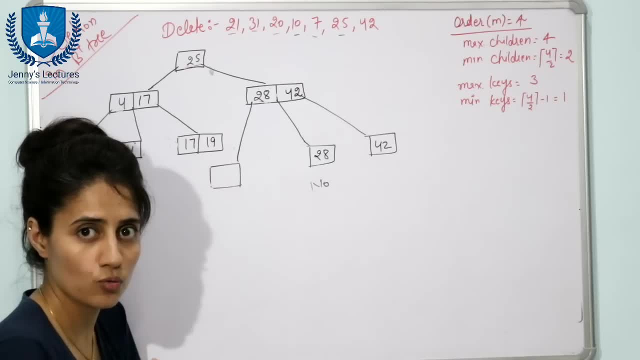 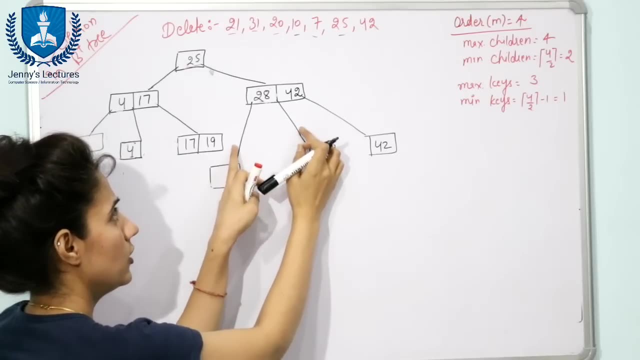 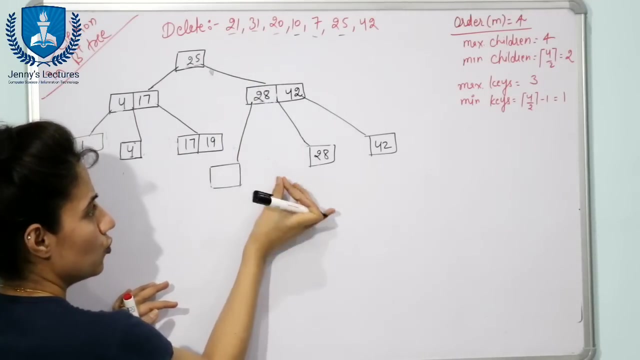 28 would be deleted. that is the rule. fine, we will merge these nodes and we will find out which which index is between these nodes and we will delete that index from the internal node. fine, so now, if you do merging of these two, so it is obviously empty. it is only 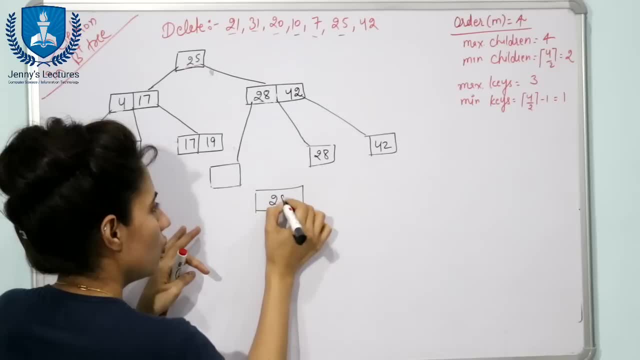 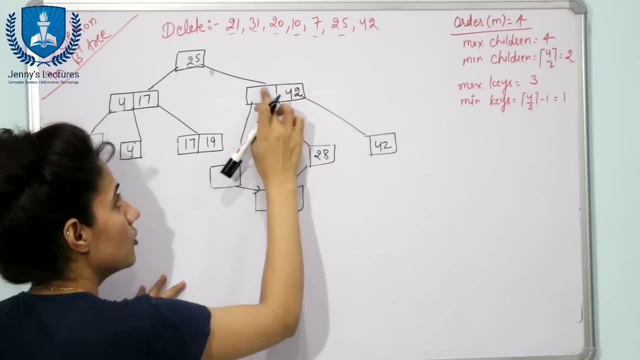 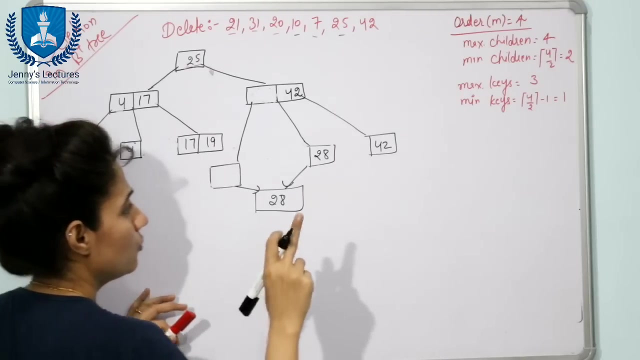 of 28, so the merging would be: we are having, finally, only 28 after merging these two, fine, and the data should be deleted from here. this 28 should be deleted from here, fine, so now. now the tree would be something like this: we don't have this. 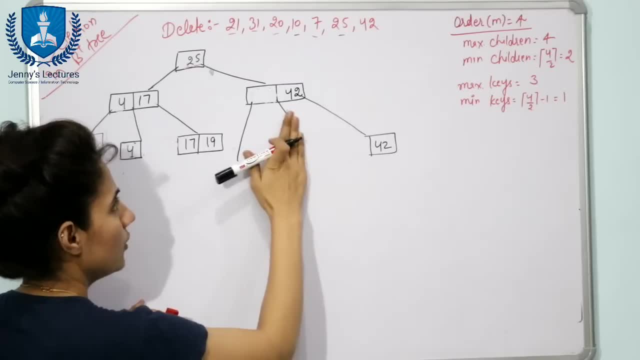 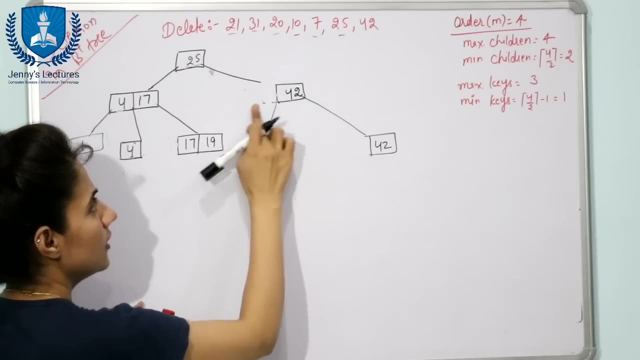 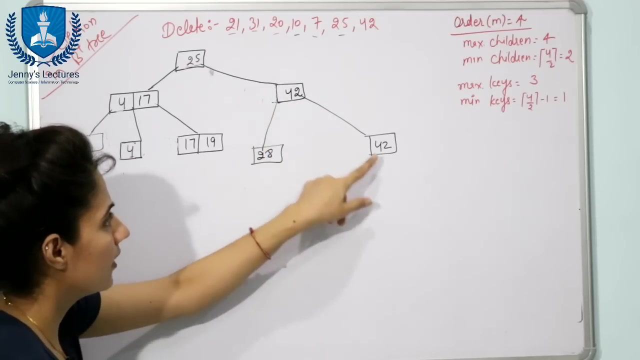 data. now we have merged these two, we we are only having one child here, only 28, and we have deleted this 28. so in this internal node also we are having only one key, that is, 42. to the left of 42 we have 28 and to the right we have only 42. fine, now, this was 25, so from here also you have. 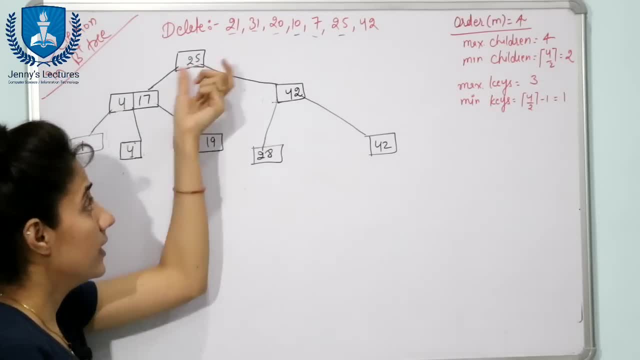 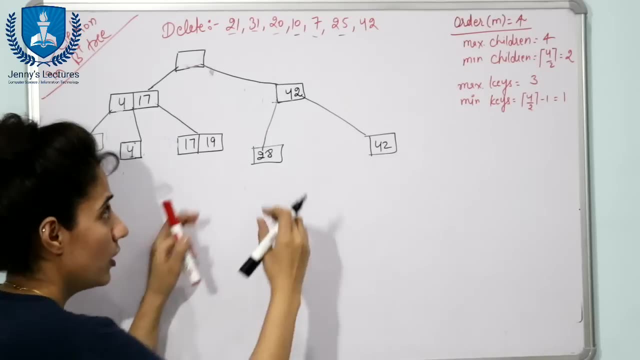 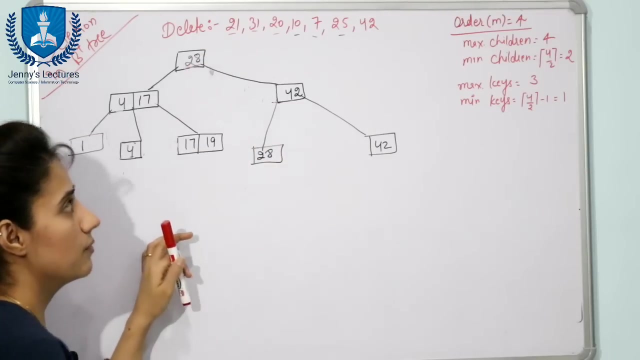 removed 25 because with the data you are supposed to delete that index also. now here you delete 25. now which value you will put here? the minimum value from its right subtree. the data is 28 and 42. only minimum is 28. so you will write 28 at this place. now, this is the tree. now next is 42. 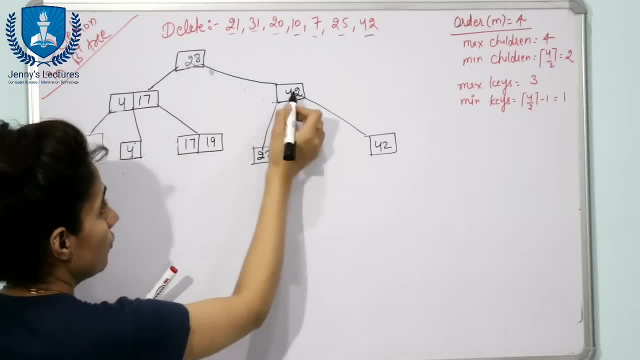 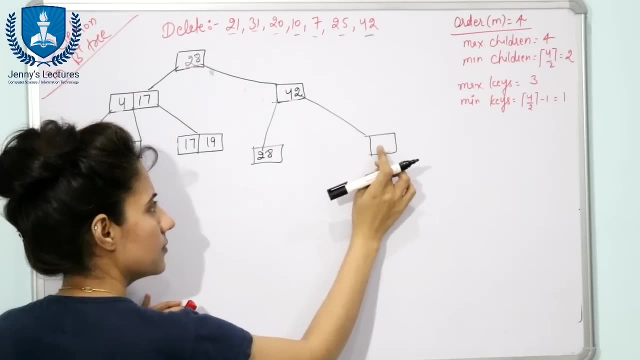 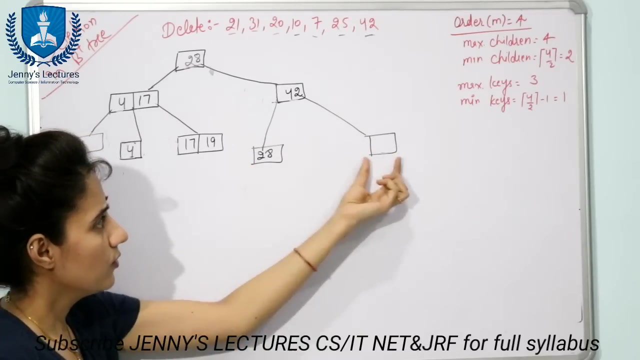 now suppose you want to delete 42. now find out where is 42 to the right of this one. this is just here. you got 42, so now delete 42 from here. check to its siblings. we this is having only left sibling. it will ask: can you give me one key? it will say no, i can't. so then merging would be done fine. 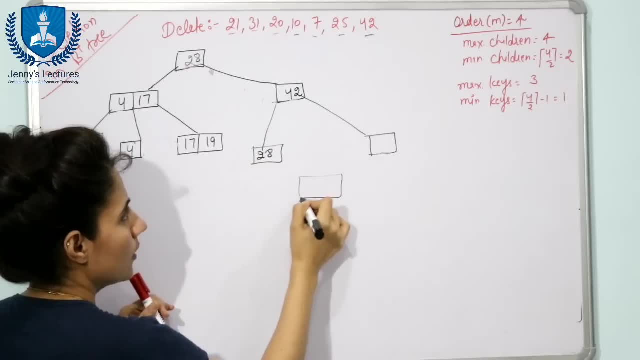 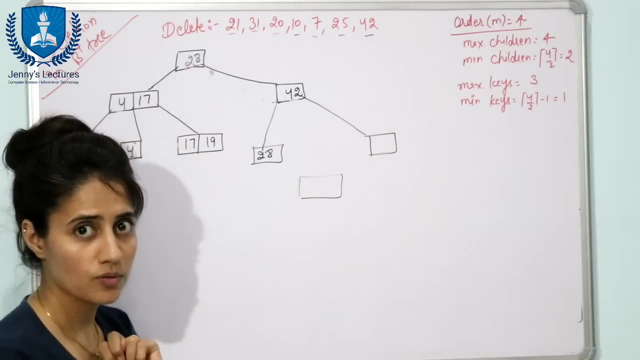 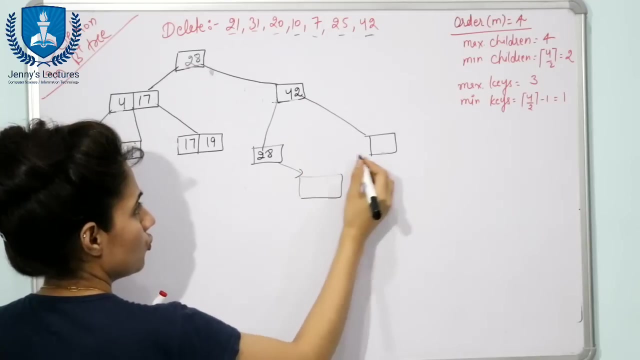 and if you merge these two, then this node is having only one child, but minimum children should be two. fine, now you what you will do, see, suppose we have deleted. after merging these two, we have only one child, that is 28, because this is the same patina. so 28 would be there now, obviously. 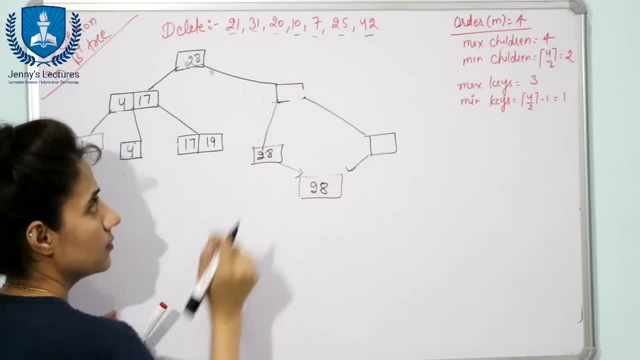 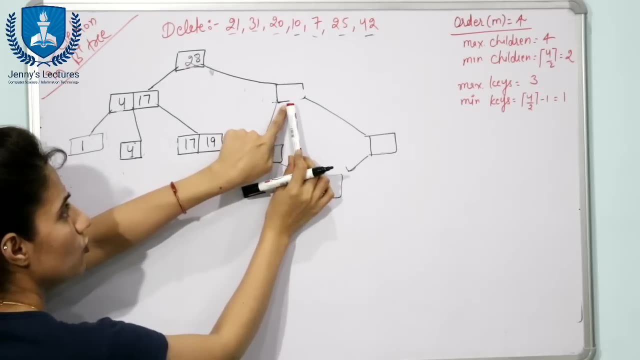 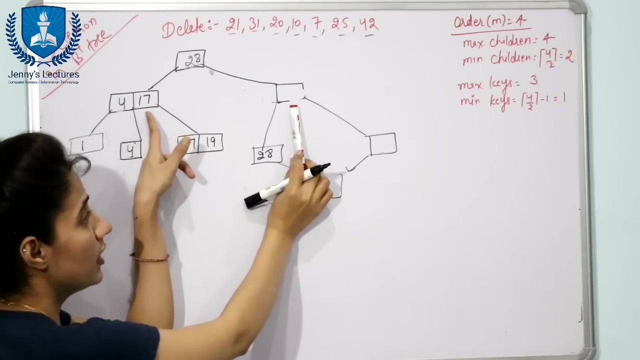 you have to delete 42 from here, right, because 42 is in this index. now, what you will do now, the same rule would be applied to this one. it will ask to its sibling: can you give me one key? it will say yes, because it is having more than minimum number of keys. now that key would be: 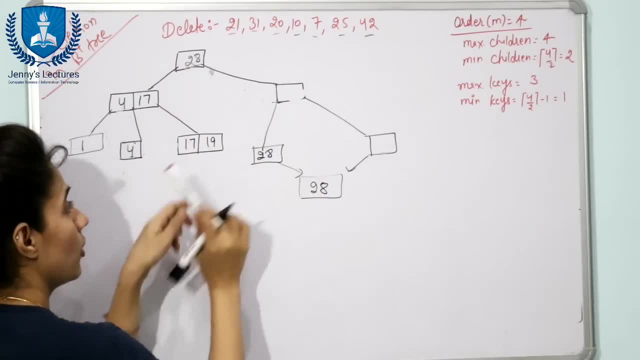 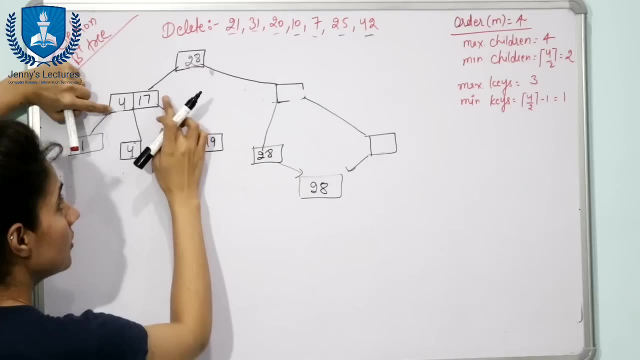 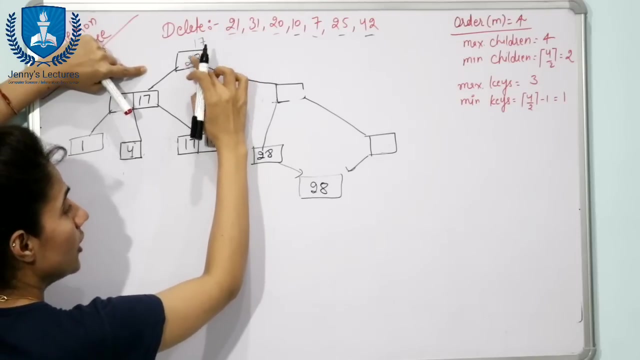 passed to this node through the parent node. now, parent is this one? now? what you will do now, what should be done from the left sibling i? i told you that the, the maximum value, would be passed. so maximum value 17 would be passed here. here, 17 would be passed and 28 would be passed here. 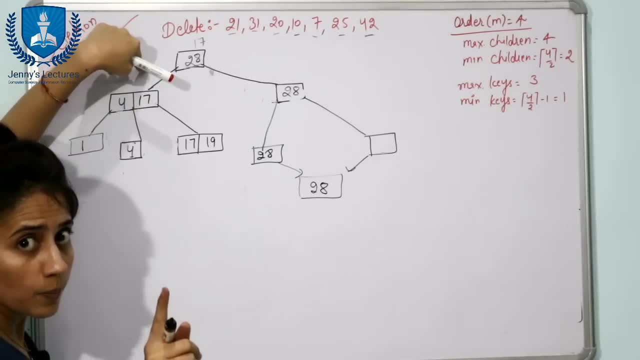 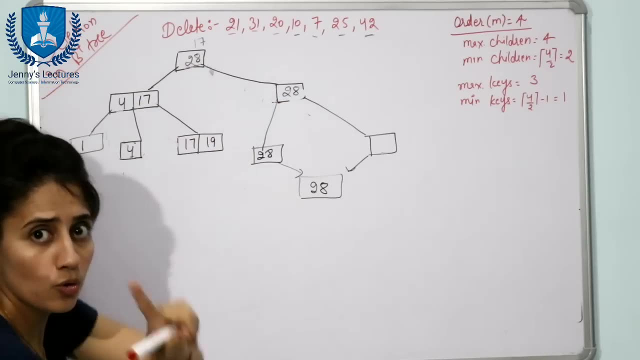 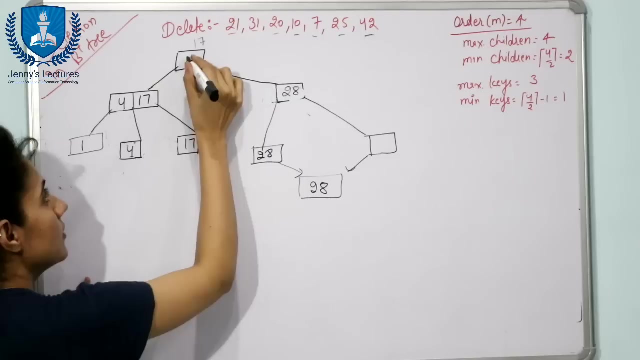 fine, because value is always passed through the root node. it's not like it can directly borrow 17 from here. no, so here we have 28, so 28 would be passed down and 17 would go up. so here you will write 17 now. now see to the right of. 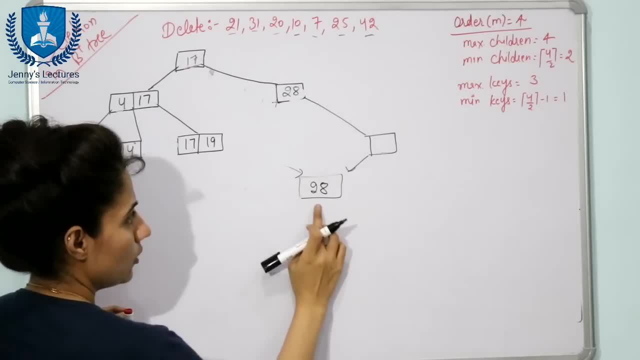 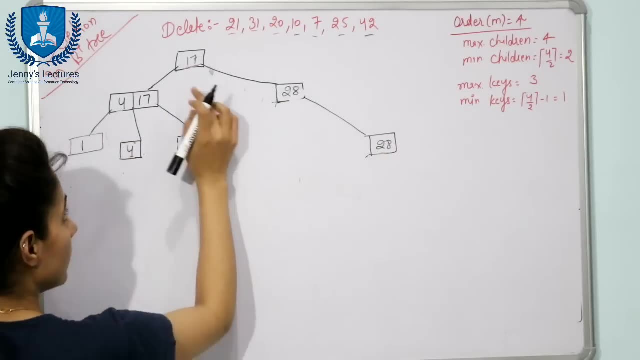 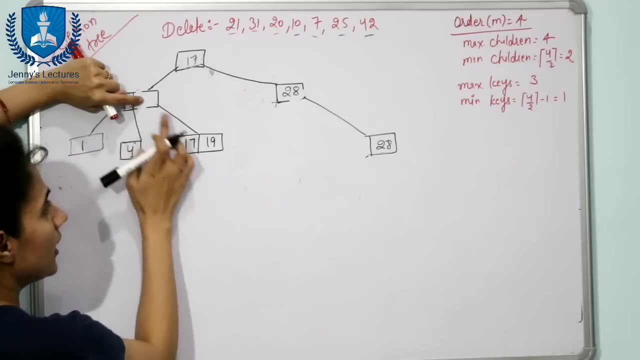 to the right of 28. see here we are having only one, one node, now 28. so to the right of this 28, we are having 28 and to the left of 28 you will have what now see. 17 would be deleted from here. so 17 deleted from here. so the right child of 17 to the right of 17. 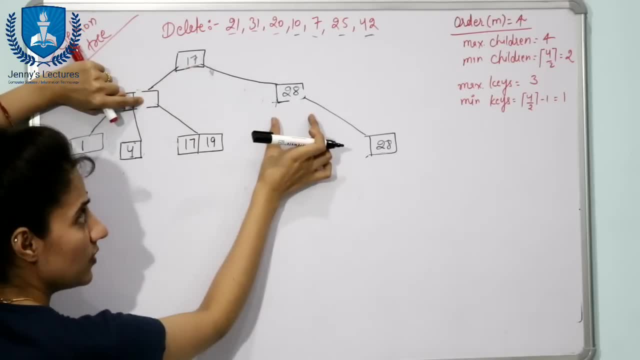 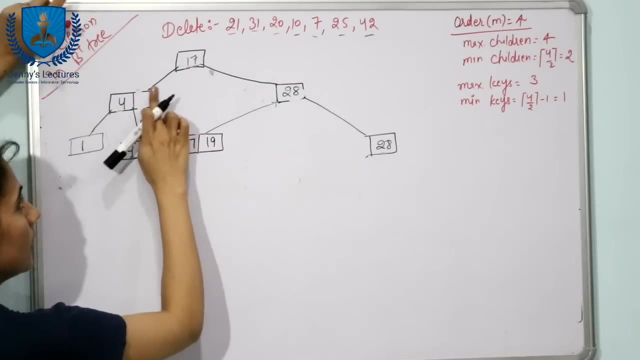 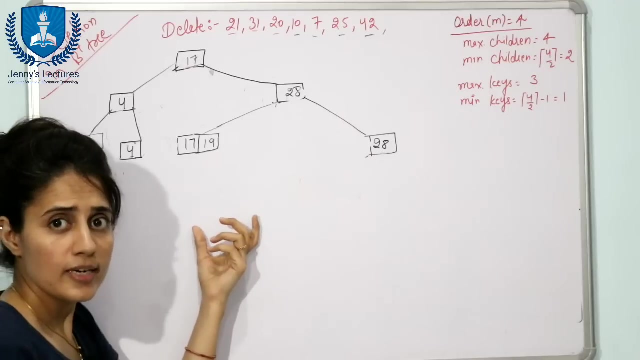 we have 17 and 19, so these values should be passed to the right of 17 and to the left of 28. so now this would become to the left of 28. here we are having only one node, four now. so now the final case is shrinking of the height. now, see, suppose i want to delete four. 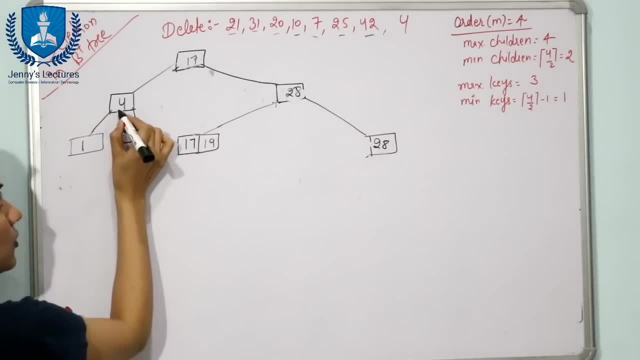 right now find out, whereas 4 less than 17. here we got 4. but this is just an index. go to the leaf node to the right of this. here we got 4. so now, if you delete this 4 from here, then it will ask to its sibling: can you, can you give me one key? it will say no, i. 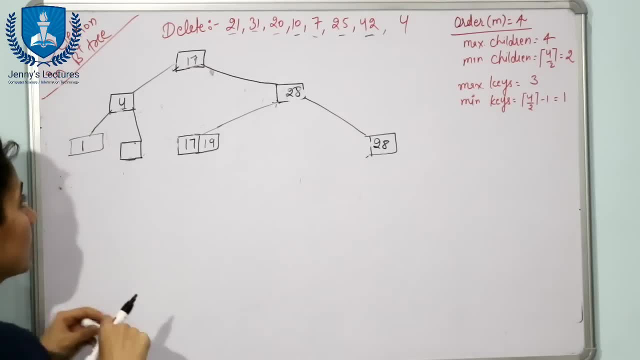 can't, because i have only minimum number of keys. in that case, merging would be done, fine. so if you merge these two nodes, then one node would be there, having only one element, that is one one. now, see, now only one, only one child is there, but that is also not possible. again, also, you have 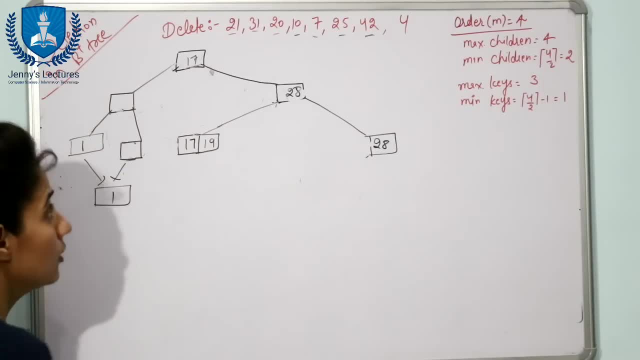 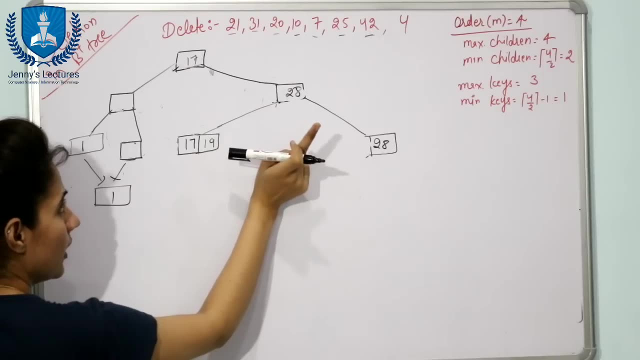 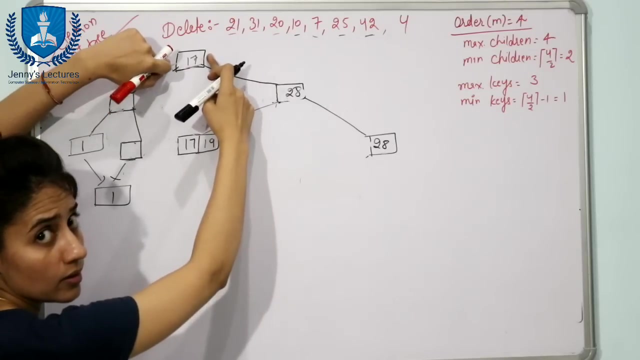 to delete four from here, right. so now this will ask, this will ask to its sibling: same rule: can you give me one key? it will say: no, i can't give you. in that case, what will happen? these two should be merged with parent, with their parent. see, that is different in in case of internal node, if nodes 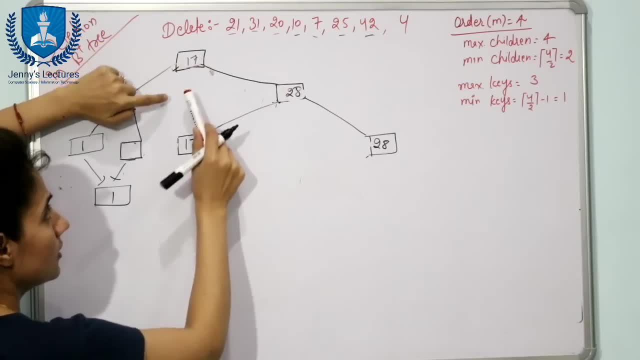 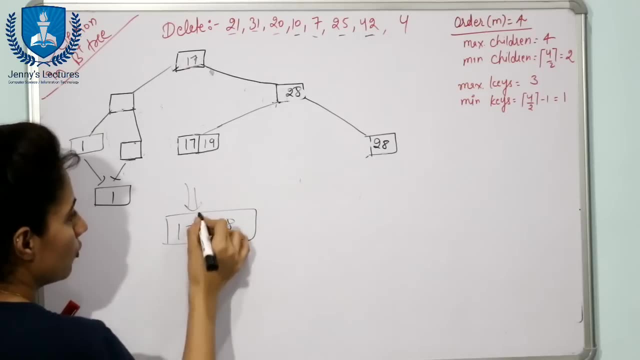 are these node to be merged with its internal node, that is, the final tree would be now 17, would go down 17 and 28 would become root. now, to the left of 17, we have only node having value 1, fine. and to the right of 17, to the right of 17 and left of 28, we have 17 and 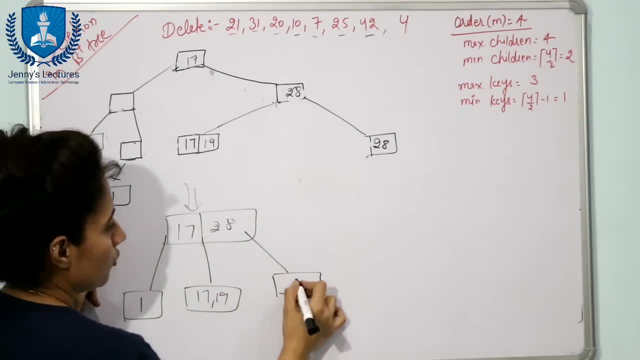 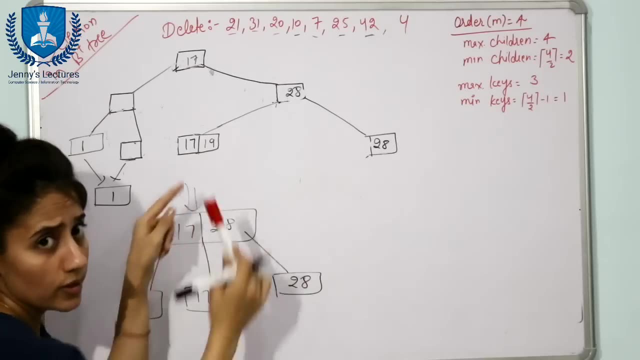 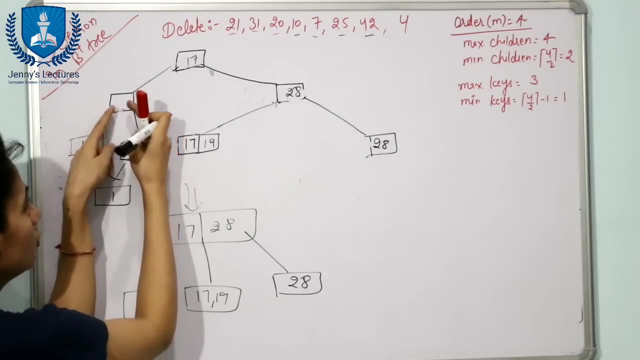 19 and to the right of 28, we are having only 28. fine, but when you are, when you are merging, when you are merging the leaf node, in that case i have told you, if you merge the leaf node, the leaf node then in between index of these nodes would also be deleted from that internal node. but in case, 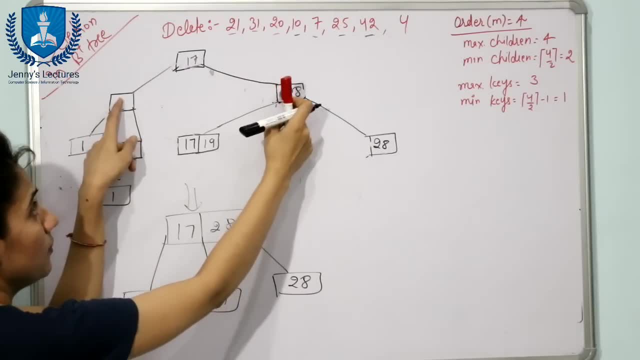 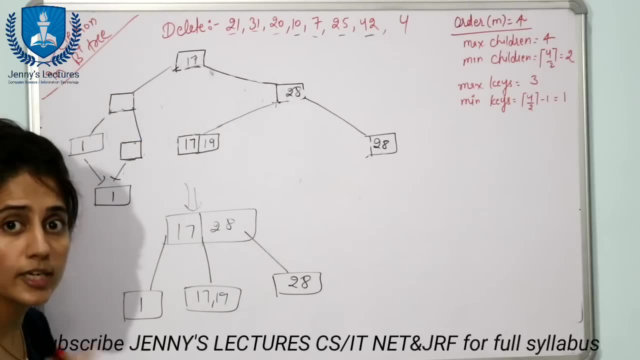 of internal node. if you are merging the internal nodes, then in between these 17, 17 would not be these two nodes in case of internal node, only fine. so this is now the root and these are the leaf node. now, fine, so this is now shrinking of the height. so this height has been reduced by one in this case. 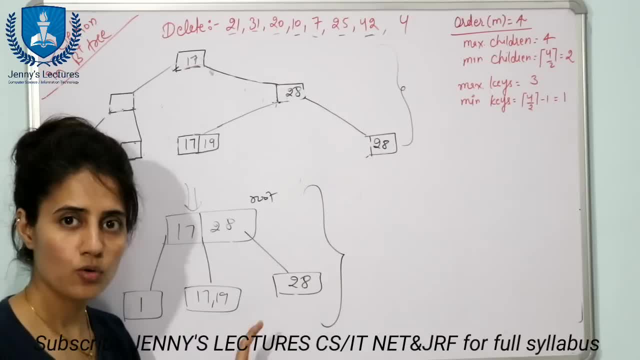 so this is how we are going to delete data from a b plus tree. i hope i have discussed all the cases, fine, so i'll see you in the next video. till then, bye, bye, take care.